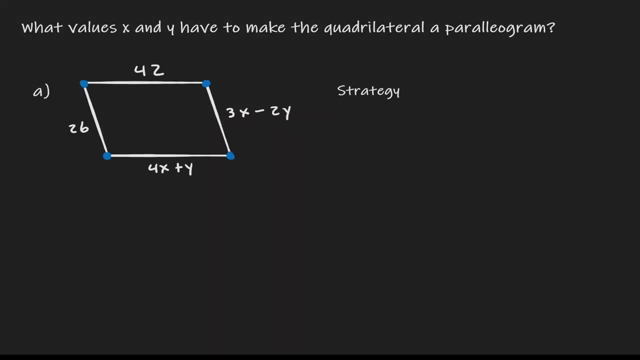 So here we have a quadrilateral and what we want to do is we want to identify what values of x and y will make this quadrilateral a parallelogram. Now let's think about strategy. If we identify where those variables are, those variables are on the side. So now let's think about what properties. 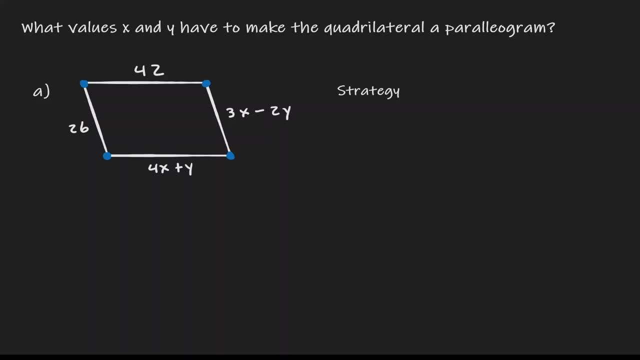 do we need to show in terms of the sides of a parallelogram. Well, we know that for any quadrilateral to be a parallelogram, opposite sides they need to be congruent. So if opposite sides they need to be congruent, then let's set opposite sides equal to each other. So here we. 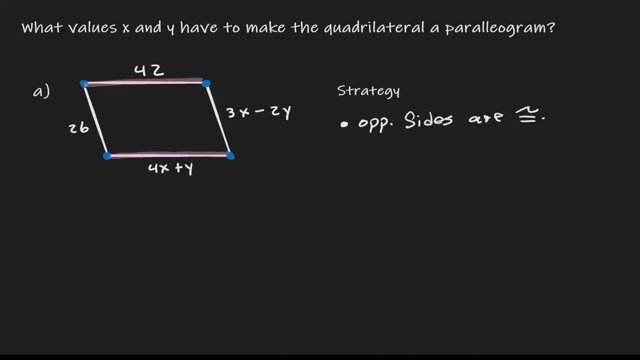 have a side of 42, and here we have a side with a length of 4x plus y. If we want them to be congruent to each other, let's set them equal to each other. So here we have our first equation. 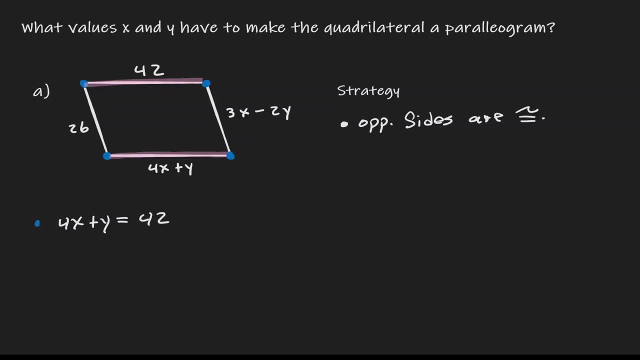 4x plus y must be equal to 42. So the same goes with the other sides. In this case our other equation, the side of 26 must be equivalent to the side of 3x minus 2y. So here we have our second. 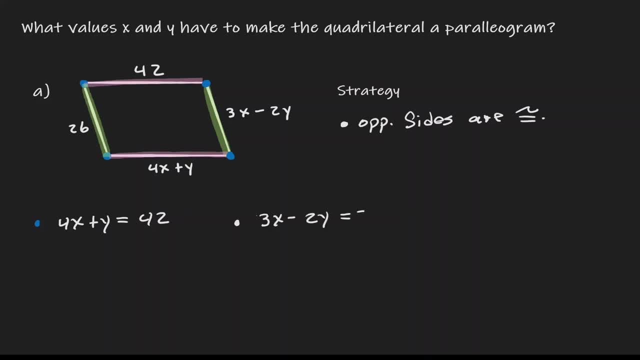 equation: 3x minus 2y equals 26.. And at this point we have a system of equations, And now we're going to think about algebra one. How can we solve the following? Well, I can see that this variable of y is kind of by itself, So let me isolate the variable of y. 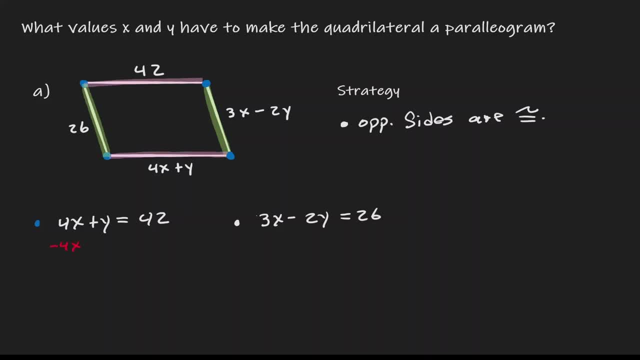 And to isolate it, let me take away 4x to both sides. So now we have: y equals negative 4x plus 42. Let me just put this on the side. And now, on my second equation, let me substitute this value of y, So now we got 3x minus 2. 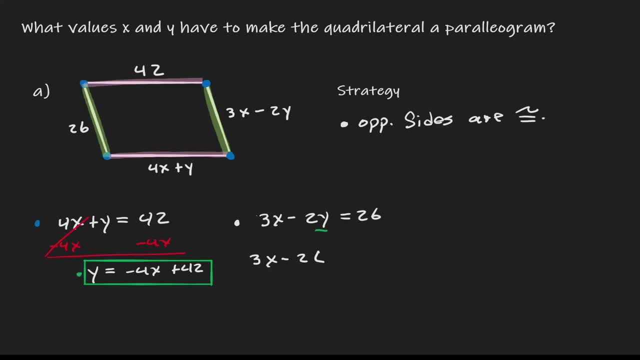 plus 42.. And now that I see that I have a y in here, let me substitute the value of y that I have here, So that will be minus 4x plus 42, plus parenthesis equals to 26.. So now let's continue. 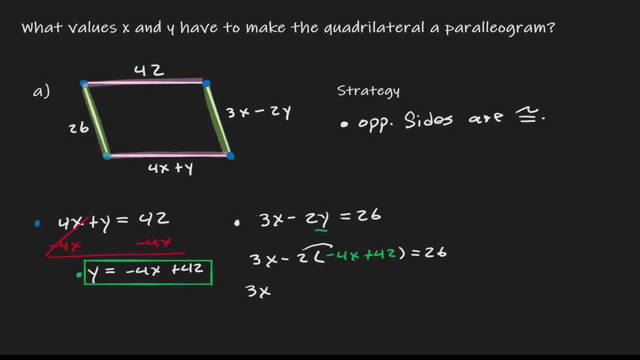 by distributing the following. So we got 3x. If we distribute now, we're going to get positive 8x, And if we distribute one more time, we're going to get negative 84 equals to 26.. Now let's combine. 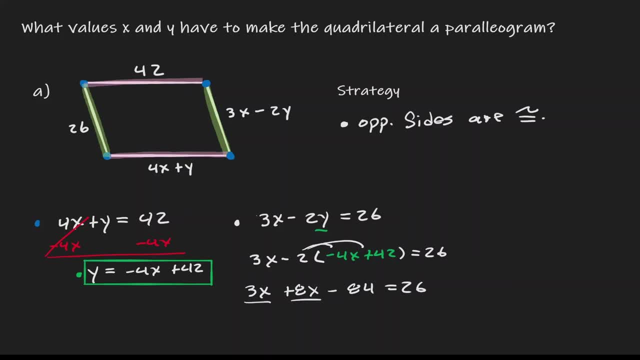 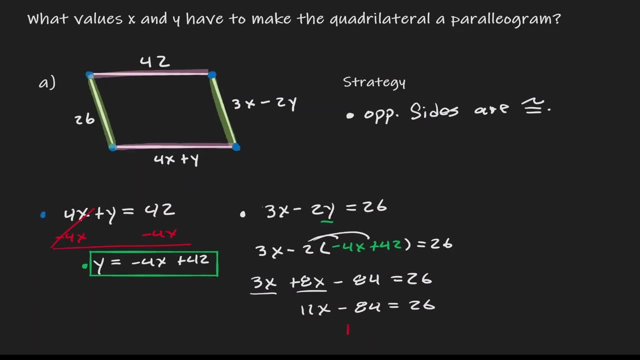 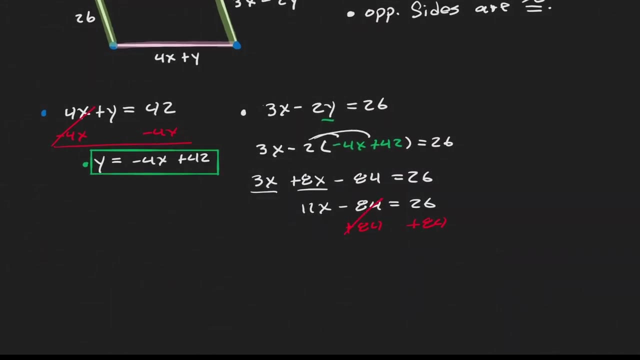 like terms. I can see that we have an 8 and a 3. So that will give us 11x minus 84 equals to 26.. So now let's add 84.. So 84 to both sides. Let's just push this down. And now we got the following: They cancel. 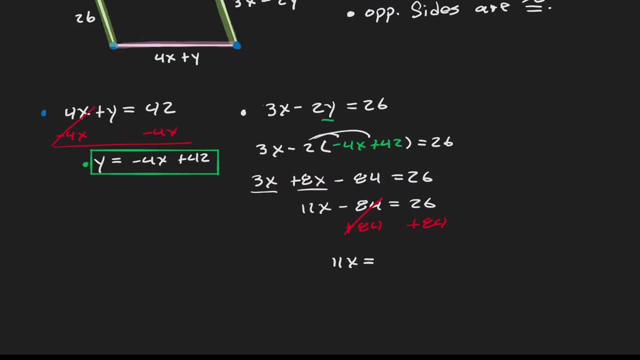 out. And now we got 11x. It's equivalent to 110.. And our last step: let's divide it by 11.. And once we have that, we can see that x has a value and that value is going to be negative 4x plus 42. So that's going to be negative 4x plus 42.. So now let's. 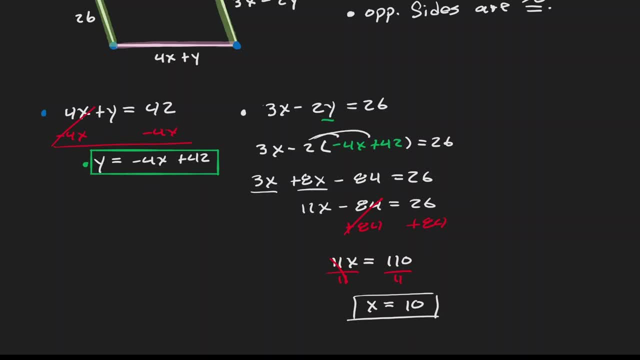 continue by distributing the following: So that will be minus 4x plus 42.. So now let's continue. We know what value of x will make this a parallelogram. Now we need to figure out what's the value of y. But don't forget, we already have an equation for y here, So let's just plug in what. 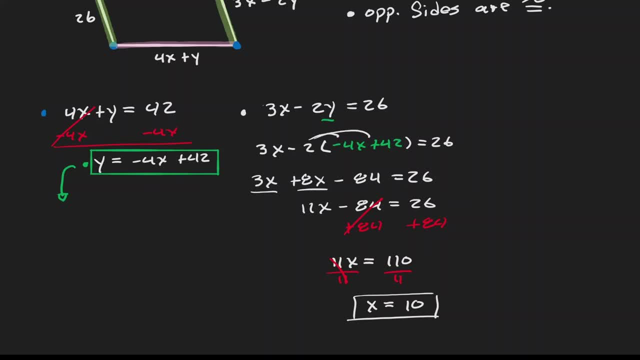 we found out for x under the equation for y, So now we have the y equals negative 4.. But don't forget x. we found out a value for it which is 10.. So let's plug it in there, So parenthesis. 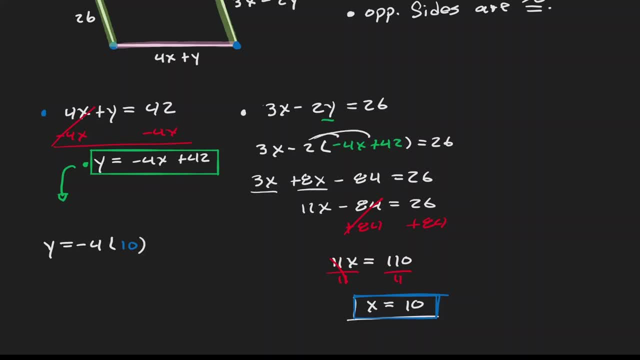 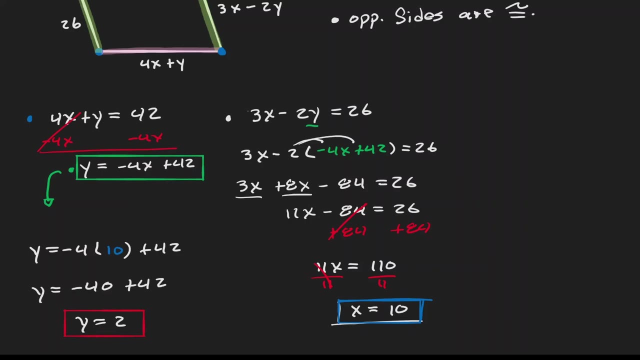 let's plug in a 10 in there, and now we got plus 42, and now this becomes negative 40 plus 42, which gives us a value for y of 2. so let's understand our conclusion in here. so we are saying, if we take a look at this, 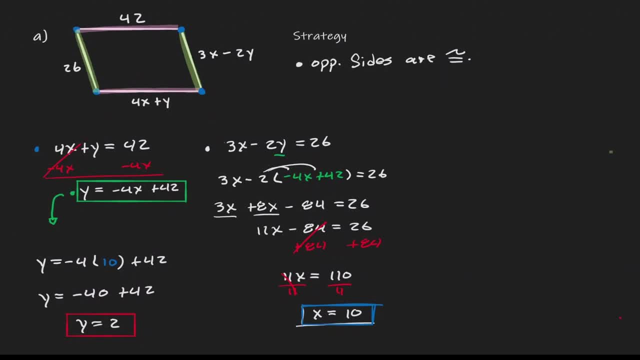 quadrilateral, and if we let x equals to 10 and we let y equals to 2, we are ensuring that opposite sides are going to be equal to each other. and if opposite sides are equal to each other, then we can label this quadrilateral as a parallelogram. let's take a look at another example here. 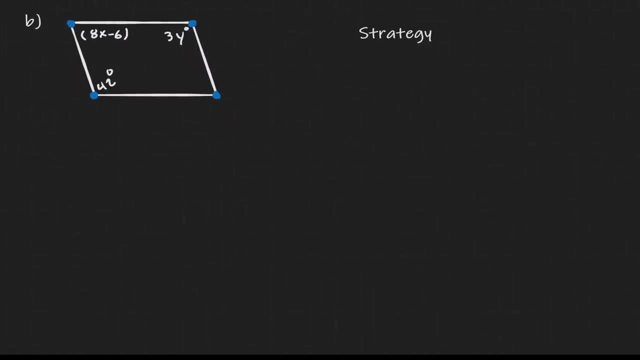 now let's think about how we're going to approach this problem. if we take a look at the givens here, every single expression are in terms of angles. so now, in terms of strategy, let's think about the different properties that we have to show for angles. well, we know that opposite. 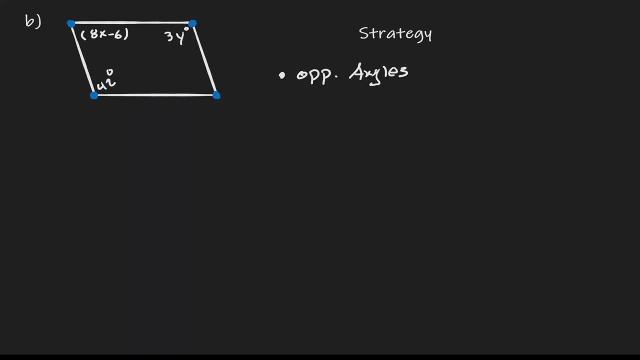 angular, LAURA angles are congruent And, in addition, we know that adjacent angles are supplementary, So let's use that. I mean, if angles, if opposite angles have to be congruent, then we know that this angle that we have here must be equivalent to this. 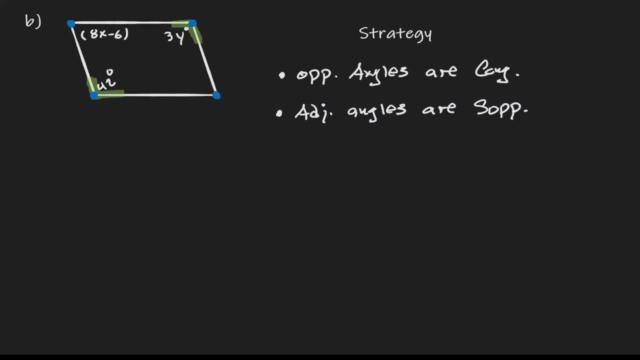 angle that we have here. So let's set them equal to each other. So now we have that three Y is equal to 42. And at this point we can solve for Y. We can divide it by three. We can divide it by three. 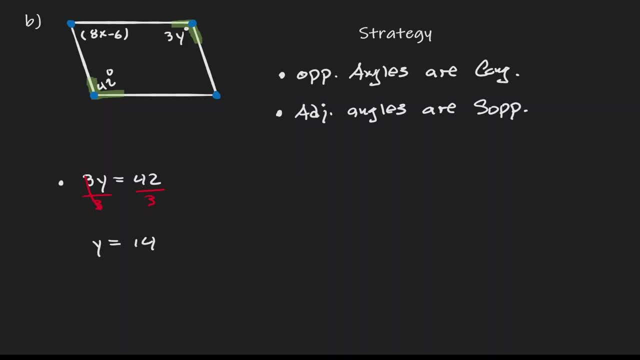 And now we can let that Y have a value of 14.. If adjacent angles need to be supplementary, then we can see that this angle that we have here has an expression of eight X minus six. it's adjacent to the angle that we have. 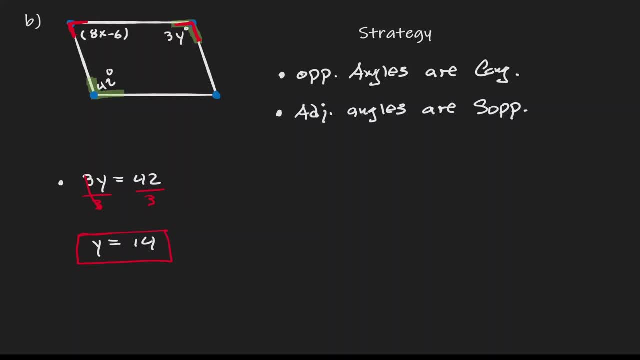 here, which has an expression of three Y. If we add them, they need to be equivalent to 180 degrees. So let's write that down. That implies that three Y plus eight X minus six, that's equivalent to 180 degrees. But don't forget that we already know what the value of Y is. 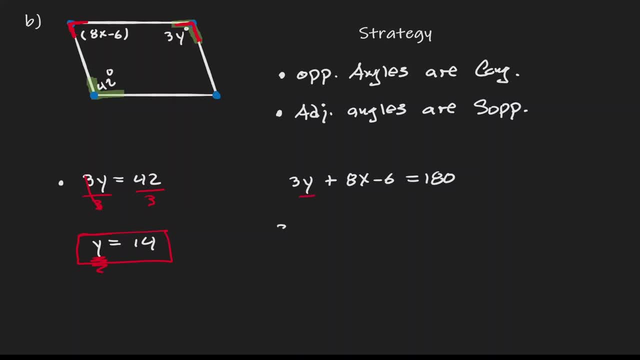 So we can just substitute that in here. So now we're going to get three times 14.. 8X plus 8, X minus six is equivalent to 180 degrees. So now that we distribute, that is 42. So now we get 42 plus eight. X minus six equals to 180 degrees. 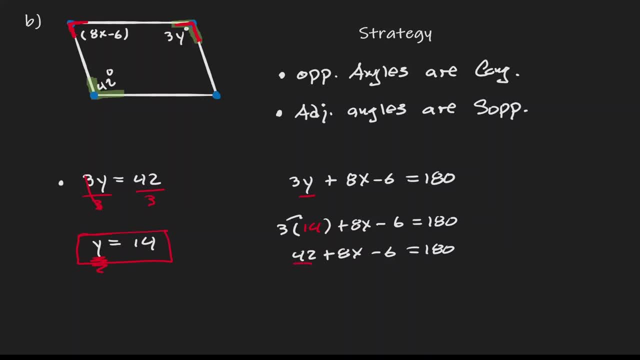 We can combine like terms now: 42 minus six, that is equivalent to 36.. So now we've got eight: X plus 36 is equals to 180 degrees 180, and notice that that's a very simple equation. let's take away 36 to both sides. 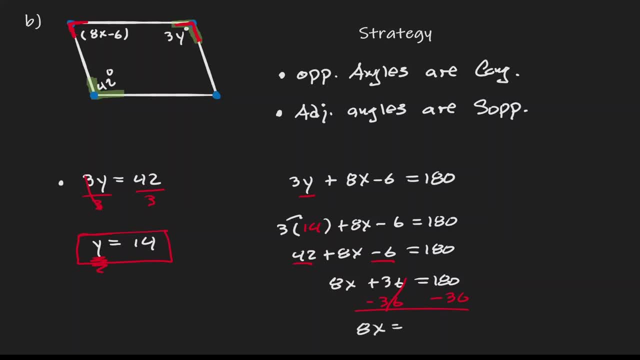 so now we got that 8x is equivalent to 144 and at the end, if we divide it by 8, now we got a conclusion, and that conclusion is that x has a value and that value is of 18.. Now let's make sense of what we have done here. we were given a quadrilateral and now we found out.